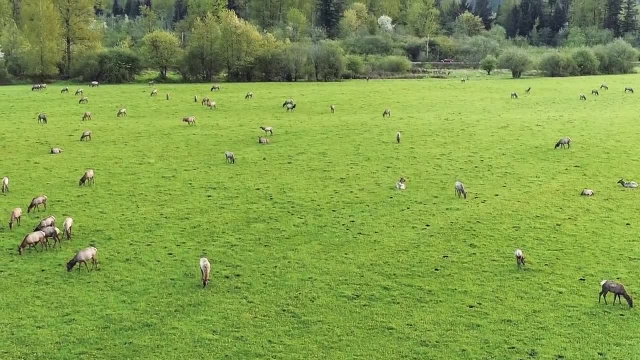 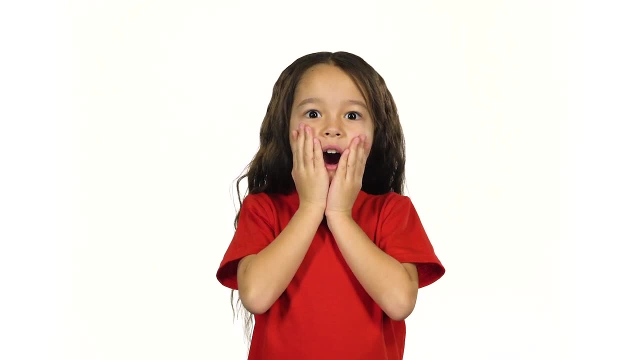 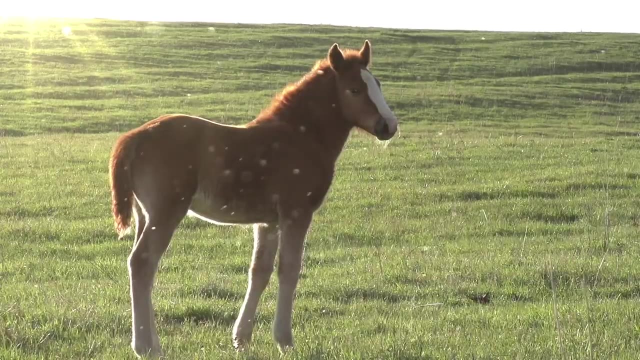 Mammals are one of the largest animal groups on the earth. All mammals have backbones or spines. A human is a mammal. You are in the same animal group as dogs, rabbits, whales and many others. Mammals are warm-blooded. 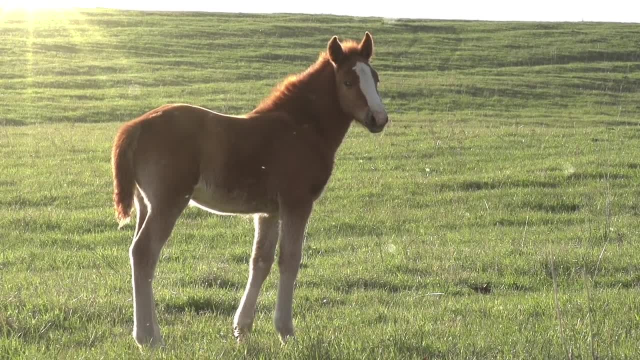 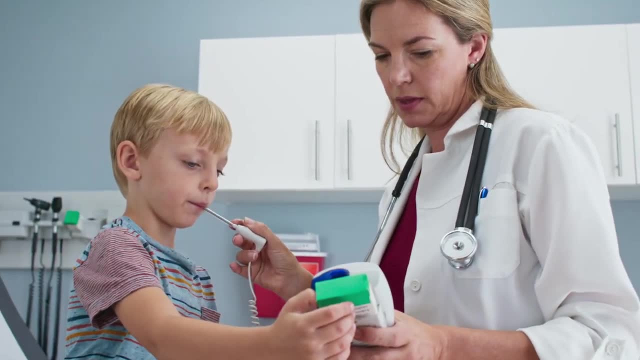 That means their bodies will always be warm-blooded. Mammals will always try to keep a constant temperature on the inside, no matter the temperature around them. Your body temperature averages 98.6 degrees, unless you're sick and have a fever. 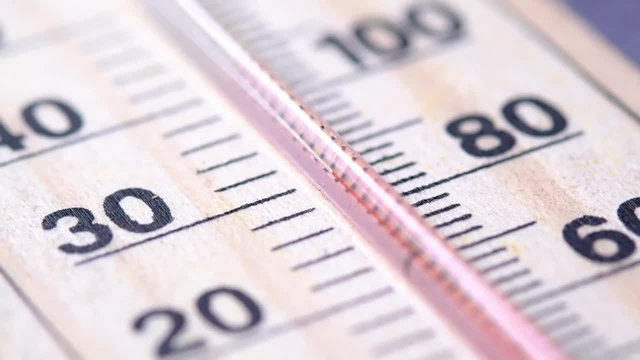 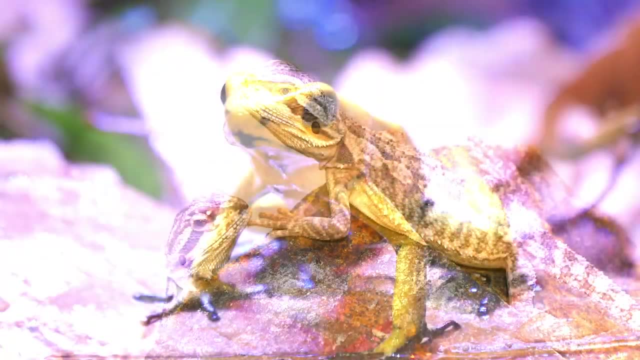 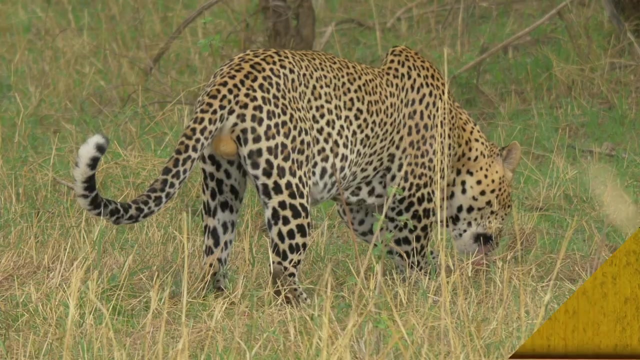 Other mammals' body temperatures average between 97 and 103 degrees, But if an animal is cold-blooded, like fish, reptiles and amphibians, their body temperature goes up and down depending on the temperature around them. Some mammals only eat meat or plants. 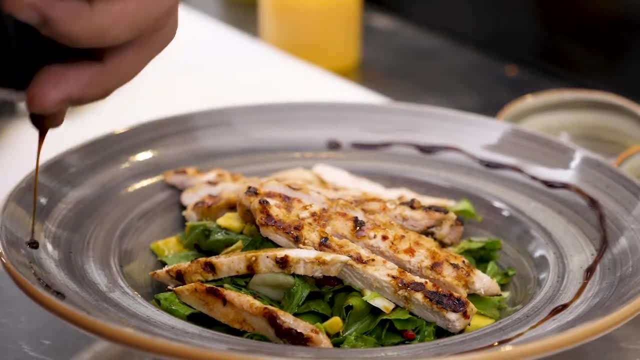 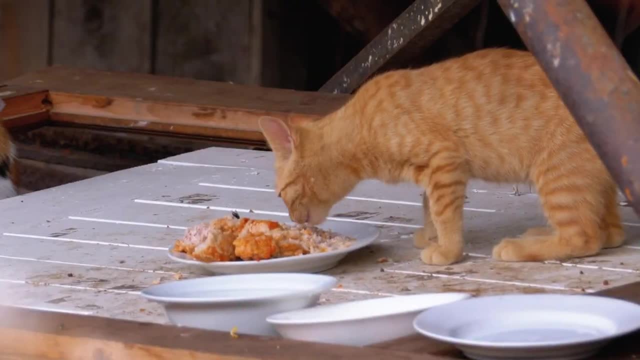 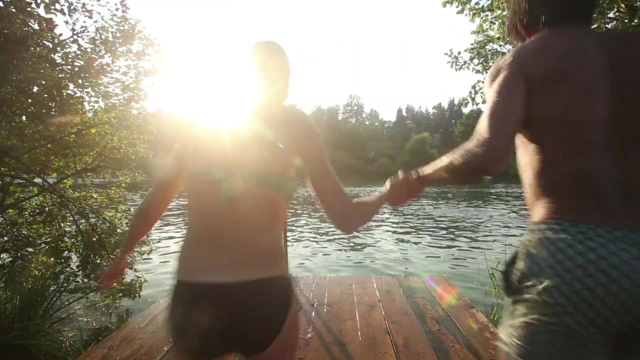 And others eat both. like humans do, Mammals generate their body heat through the food they eat, which is converted into energy. Mammals must eat more food than cold-blooded animals to allow them to maintain a constant body temperature. Have you ever jumped into a freezing cold ocean or lake and found yourself shivering from the cold? 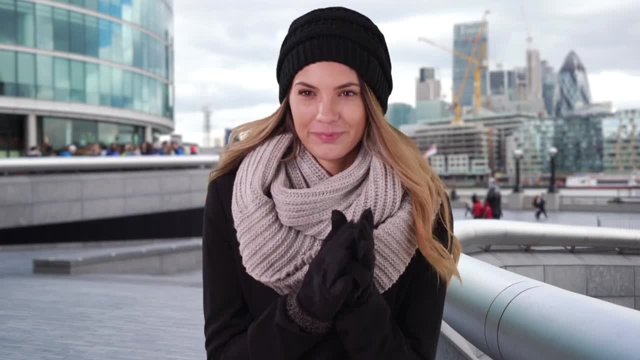 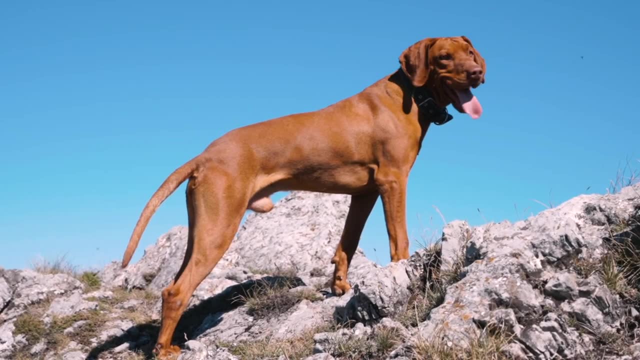 Your body is trying to warm you up and change your body temperature. Shivering generates little bursts of heat. Your body also tries to cool us down by sweating. Some mammals have other ways of cooling themselves down. A dog pants and a pig rolls in the mud. 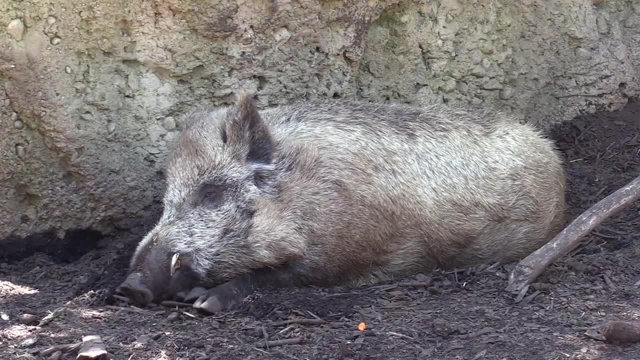 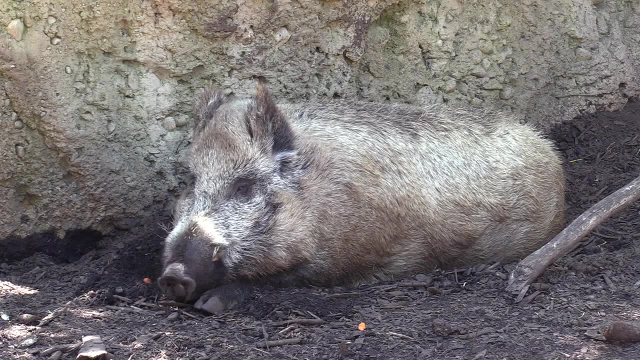 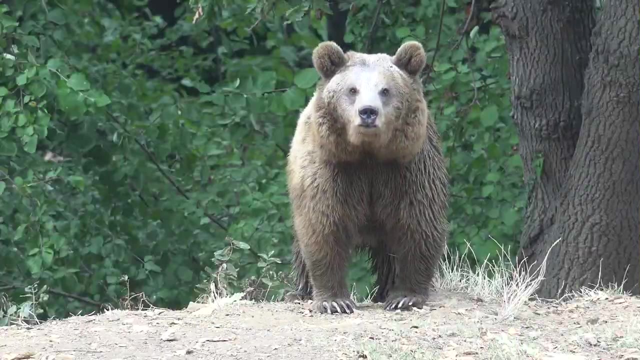 The mud protects the pig's skin from the sun, And when the water droplets in the mud evaporate, it leaves the pig's skin moist, which also helps cool it down. All mammals have hair or fur that cover their bodies. For mammals that hibernate, like bears, lemurs, squirrels- 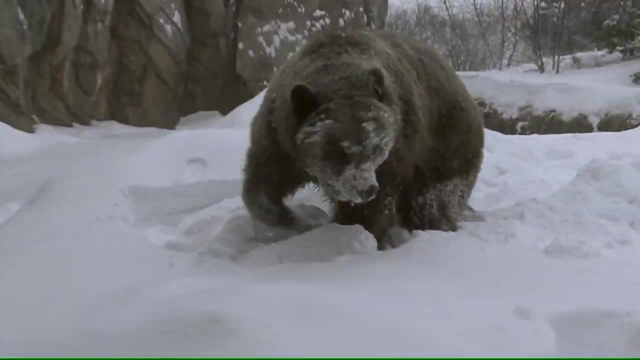 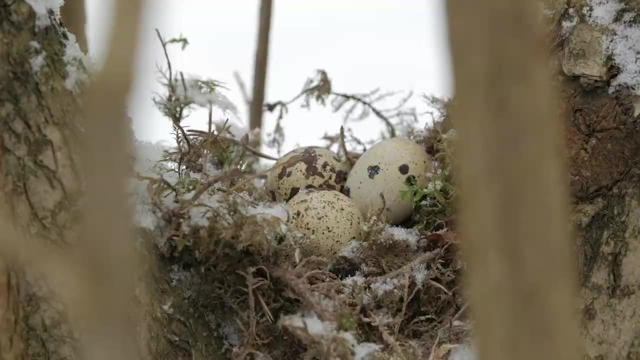 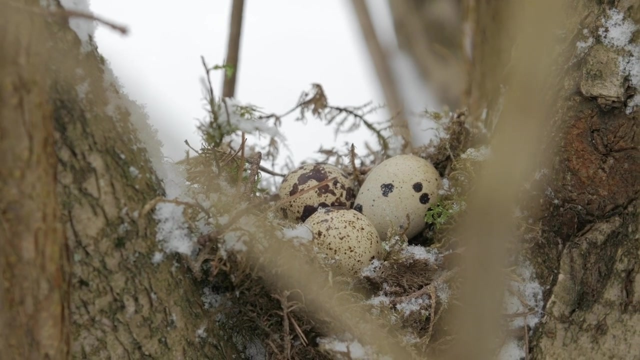 and skunks fur helps keep them warm all winter long. Another characteristic of mammals is that almost all of them give birth to live babies. This is different from fish and birds, which lay eggs that will eventually hatch. There are only two mammals that lay eggs. 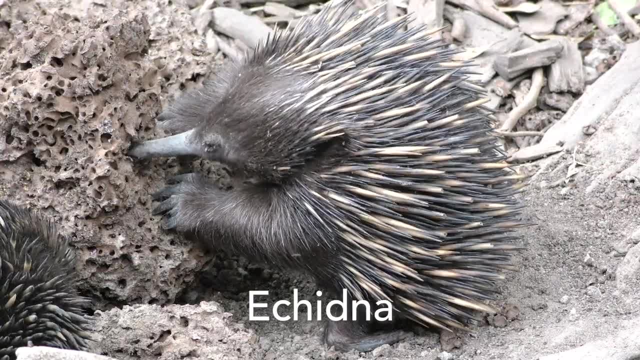 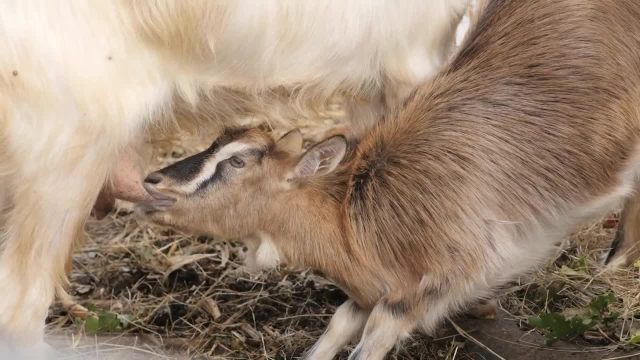 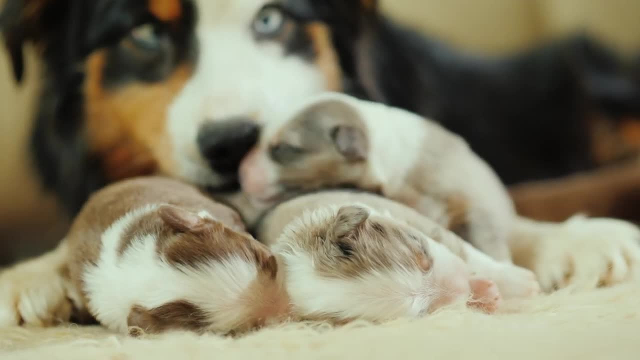 The platypus and the echidna, which is kind of a mix between an ant eater and a pug porcupine. Mammal mothers nurse their young with milk that their bodies make. A newborn mammal like a human or a puppy or a kitten needs a parent to take care of them after they're born.